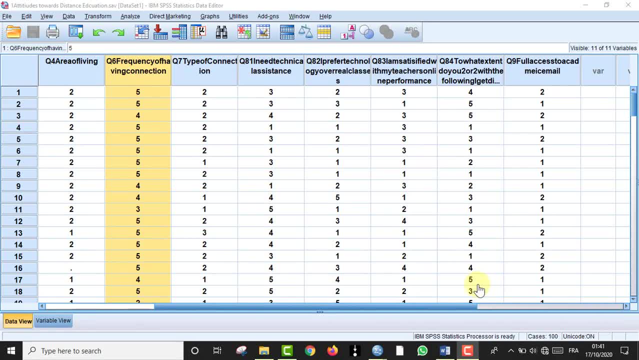 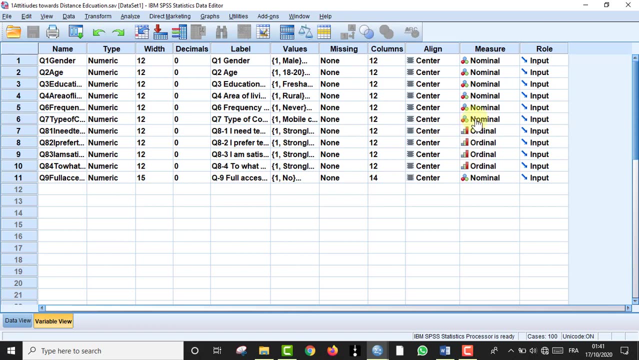 hello everyone. today I'm going to show you three ways to represent Likert scale data using a spaces. so the first way. so imagine that you have your variables entered like this and the scale or the measure is ordinal. so and this questionnaire, I have four statements in the form of five-point Likert data scale. 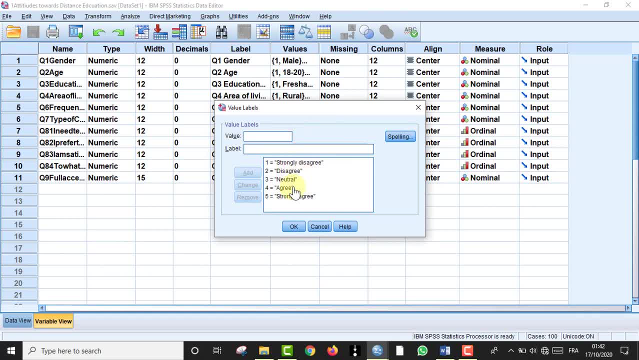 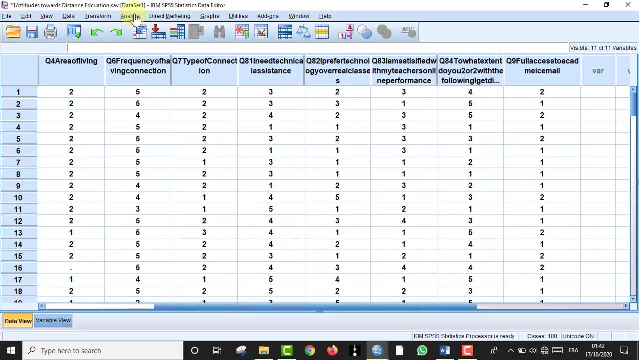 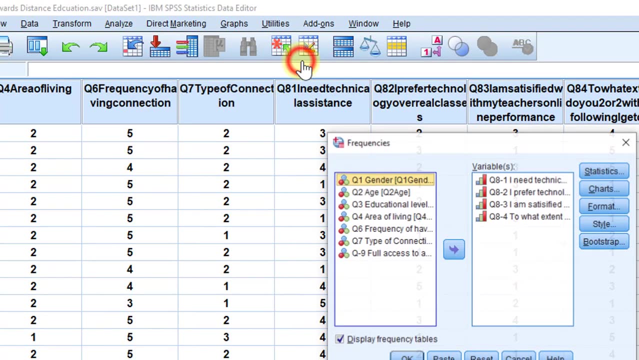 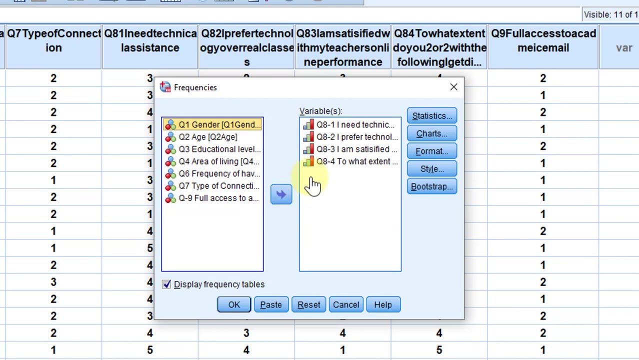 as you can see, ranging from strongly disagree one to strongly agree five. so let's go to the data view or and go to analyze descriptive statistics. so this is the first way I'm showing you, the first way, frequencies and I'm going to move the four statements in my Likert data or my Likert scale to this. 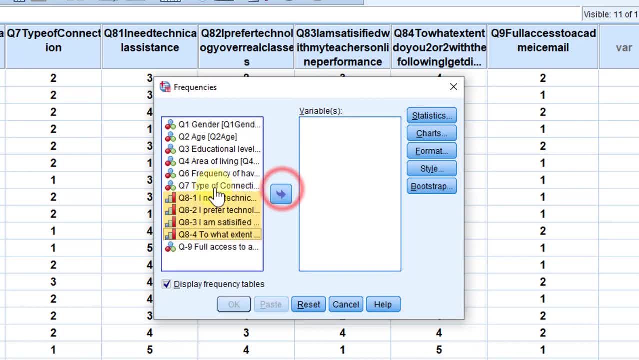 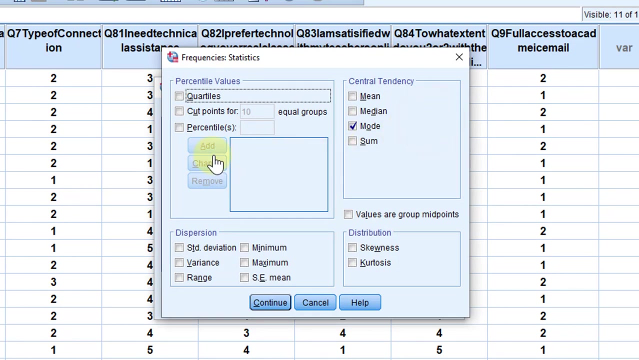 variable view. I'm just going to and do it to show you how I did that. so I just select each statement and then by clicking control and let's click in, then we move to. we click on this arrow to move the variables on the variable to the variable view. go to statistics. we leave. 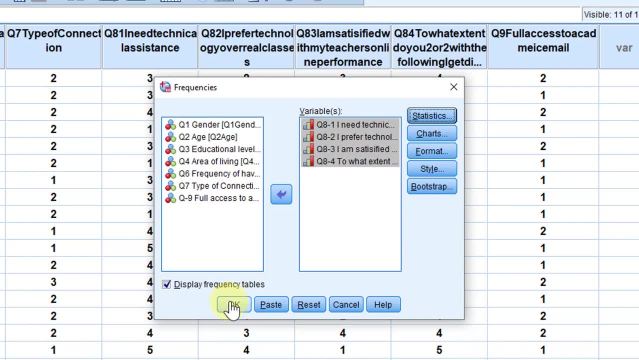 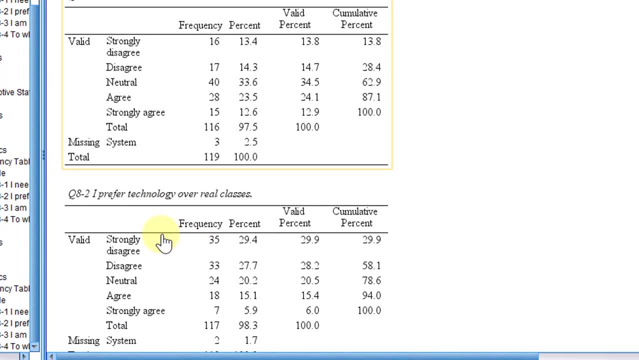 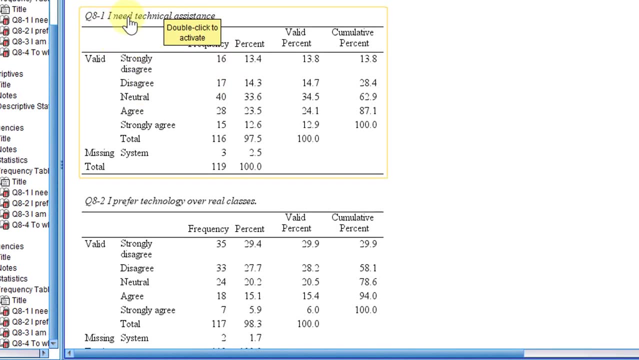 this like this: we click continue and okay. so this way it displays frequency tables. that is, we have frequency and percent. so this is the first way I'm going to take each statement and represent the frequency of each item in terms of strongly agree or from strongly disagree. 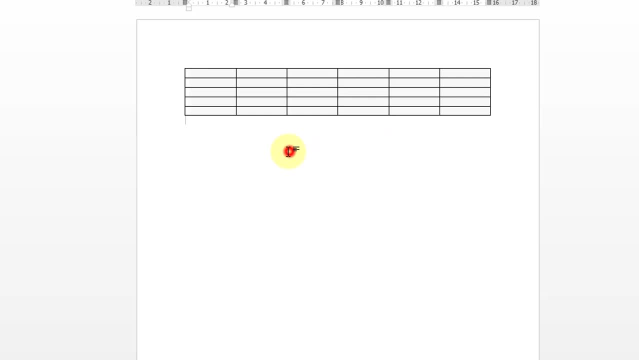 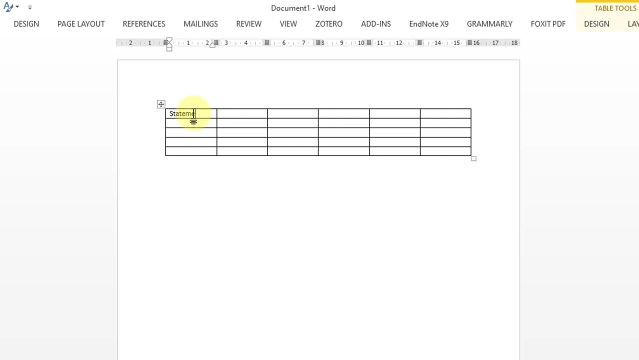 to strongly agree. so I have already created the table on words. so I'm going to put on this column statements. then I'm going to represent or write the scales from: strongly agree, disagree, strongly disagree. so then I'm going to put statements here. statement number one: let's go into zombies to show you what I'm doing. 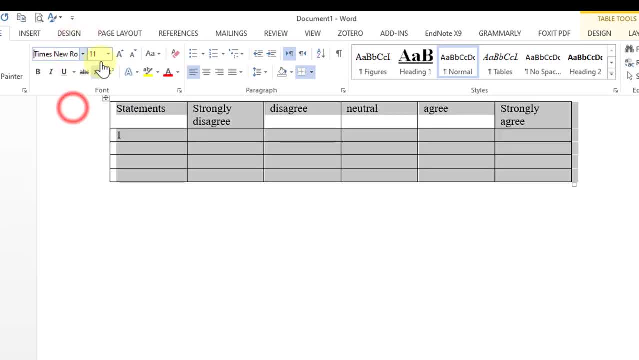 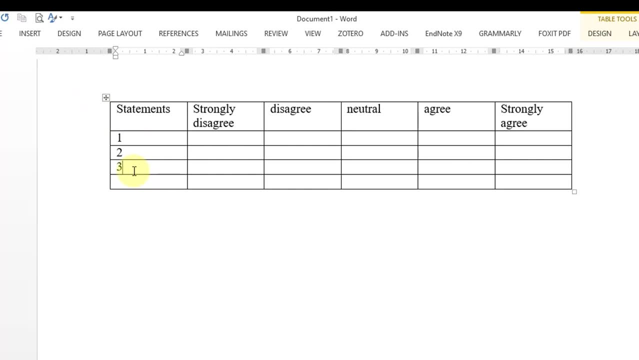 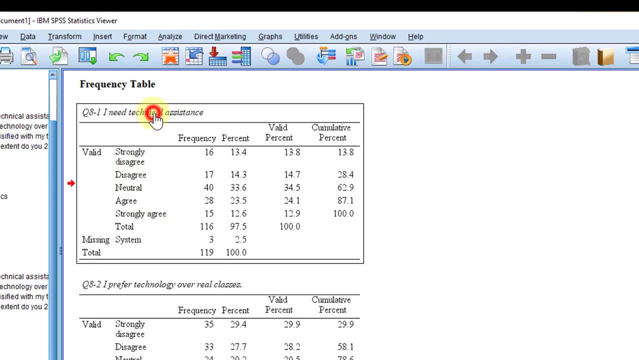 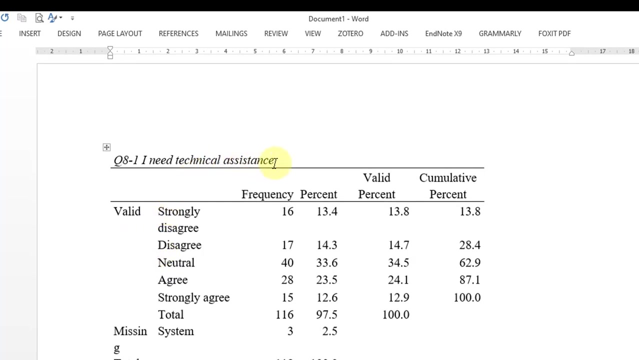 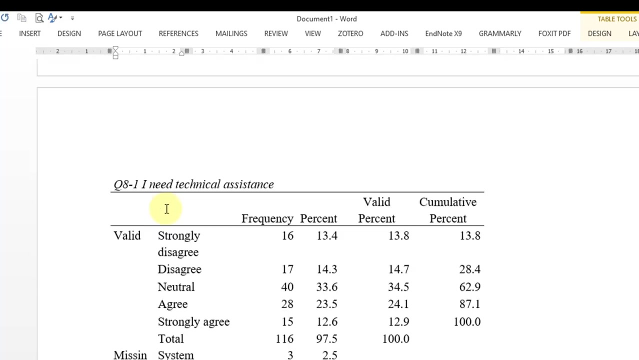 you. statement number one. statement number two. statement number three. statement number four. so then I'm going to go to the output view and look at each statements, copy and paste the table of each statement and put it. so I'm going to copy first statements. I need technical assistance and represent. 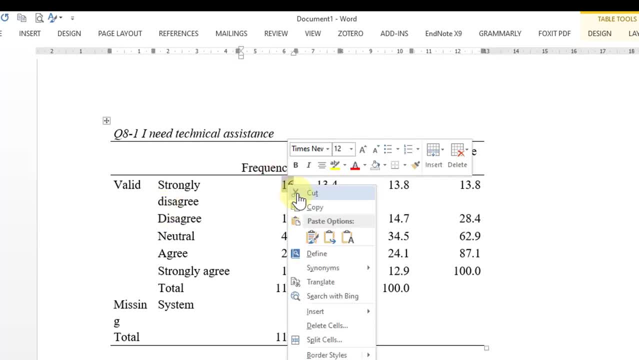 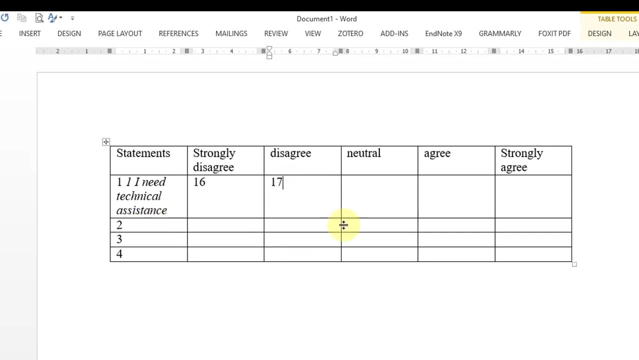 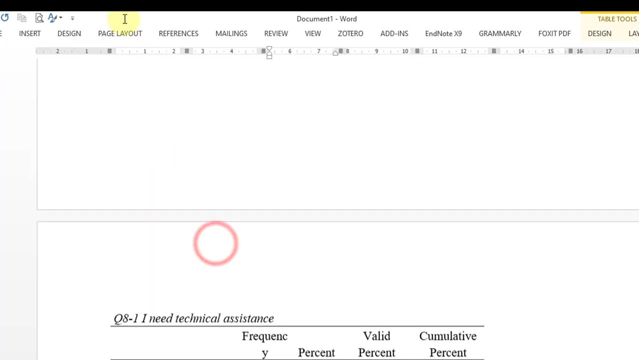 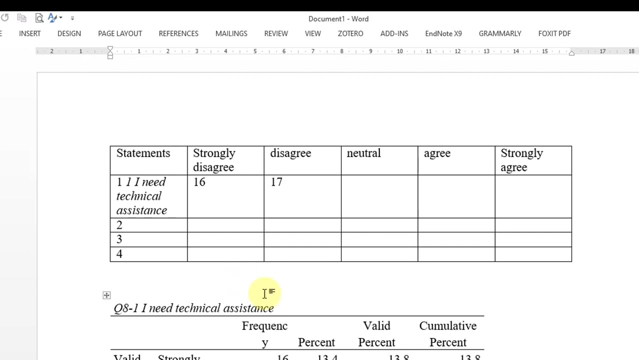 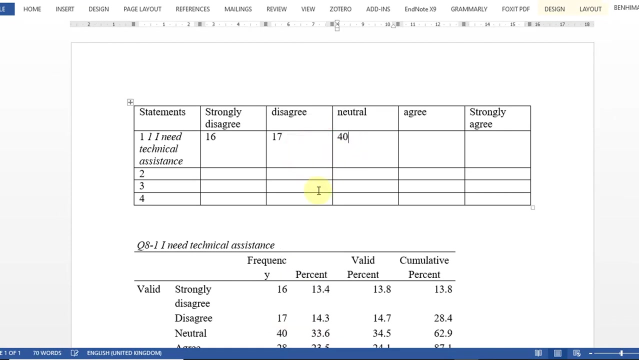 its frequency. so for strongly disagree, we have 16, for disagree, we have 17. this 17 respondents disagree with that statement. then we have 40 respondents. just going to get this here to show you how to represent the data: for neutral, we have 40. for agree, we have 28. and for strongly agree, we have 15. 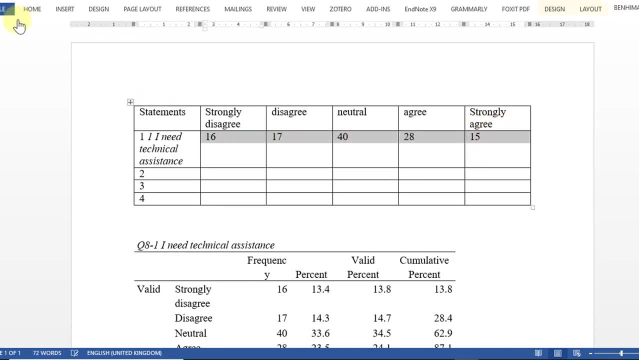 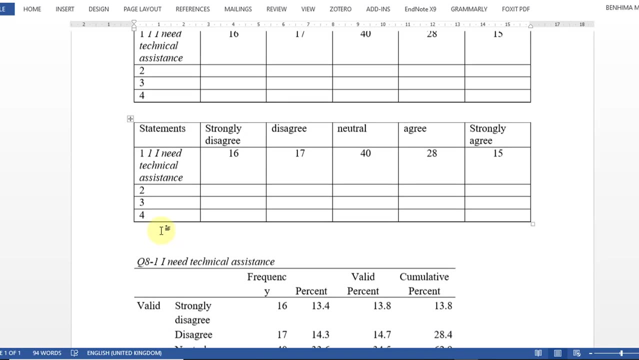 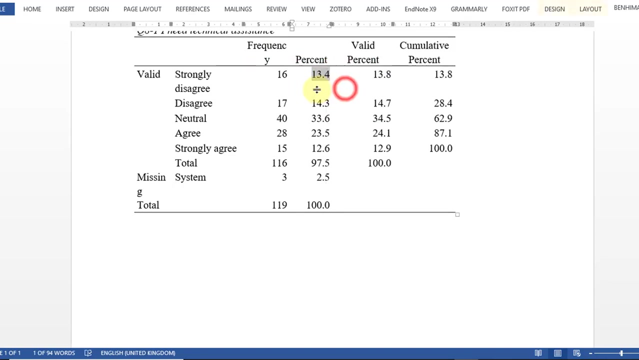 so this is the first way of frequency, and I go like this with all statements. the second way is going to be about percentage, so I'm going to use the same output, but I changed: instead of frequency I go to select percent. so I'm going to replace the frequency with the percent, like this. so this is the first way of frequency, and I go like this with all statements. the second way is going to be about percentage, so I'm going to use the same output but I change: instead of frequency I go to select percent. so I'm going to replace the frequency with the percent, like this: so this is the first way of frequency, and I go like this with all statements. the second way is going to be about percentage, so I'm going to use the same output but I change: instead of frequency I go to select percent. so I'm going to replace the frequency with the percent, like this: 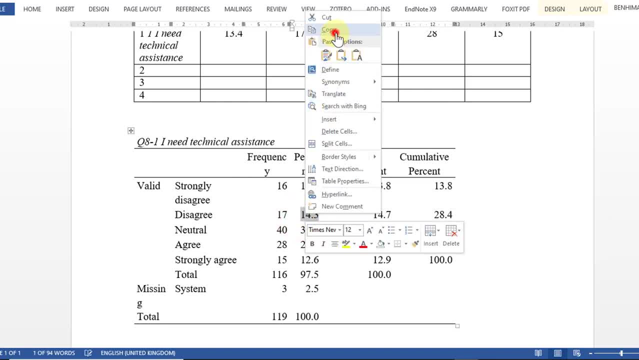 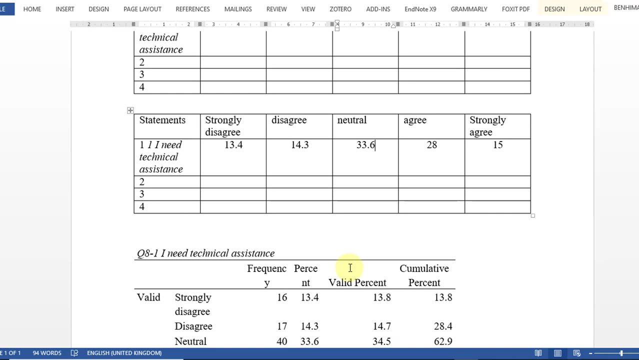 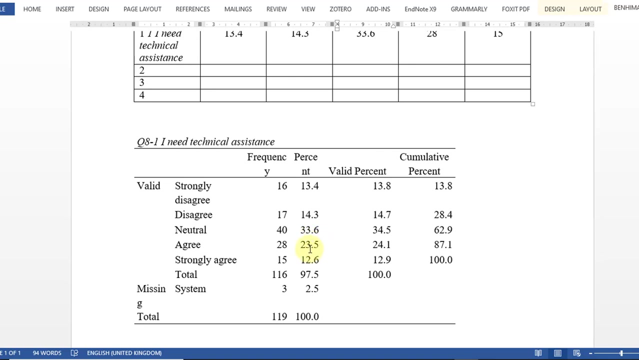 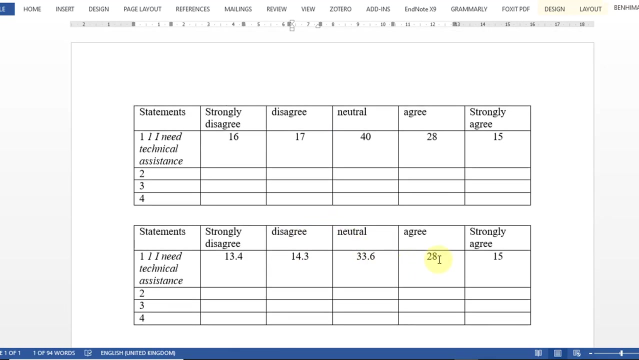 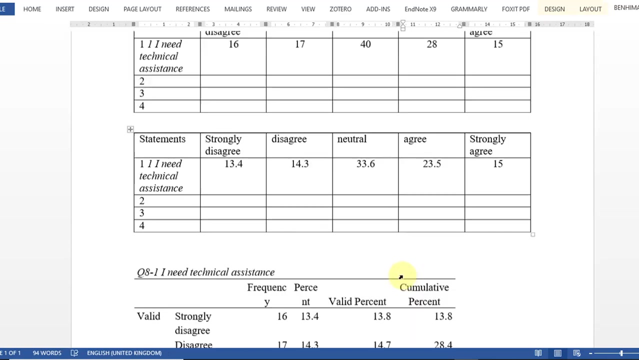 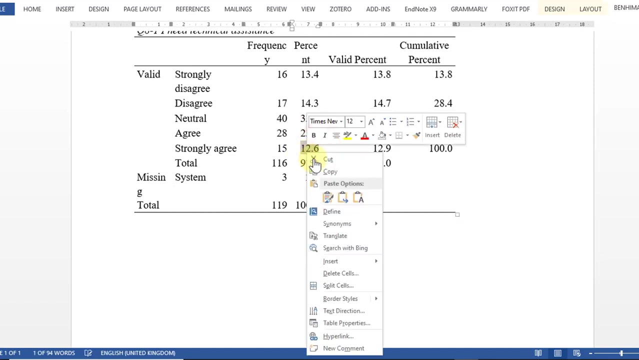 this. as you can see, you can follow me step by step. if you have your data with you and you want to write the report, try to do this. you choose either way, whether you choose frequency or persons. if you have small number, frequencies are recommended. what with larger, with large numbers, percent is recommended. I'm just 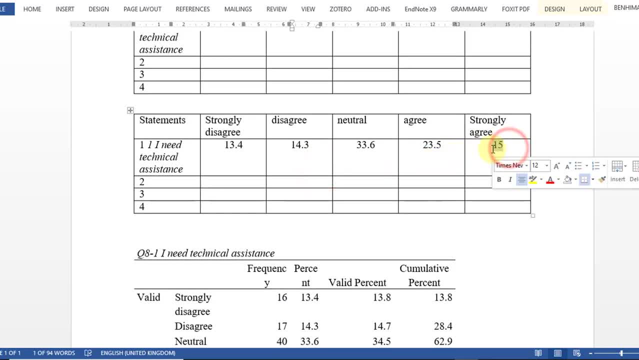 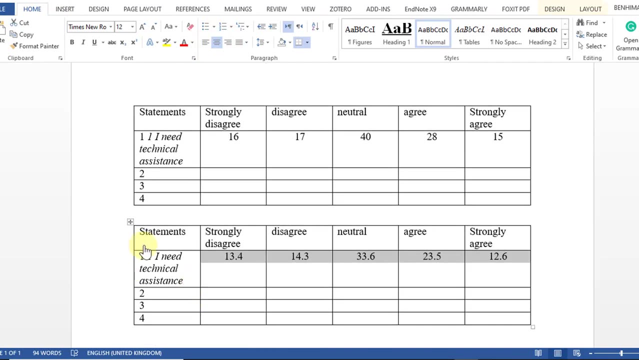 sharing with you this method because I have seen it in some peer-reviewed journal articles. I'm sharing it with you. so this is the first order. this is the second method, as you can see. so, from one output, and I can go like this with all statements. okay, then we are going to move to the show. 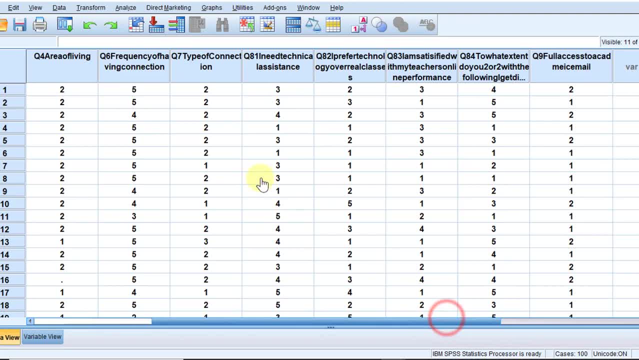 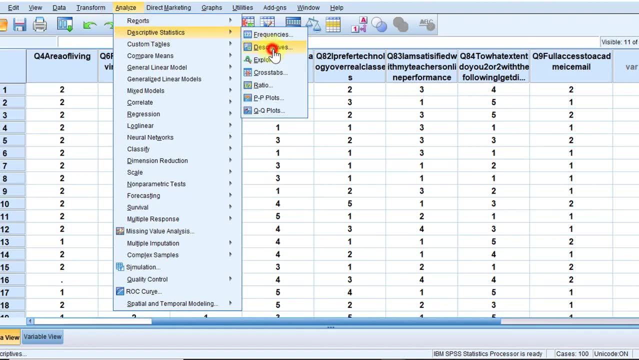 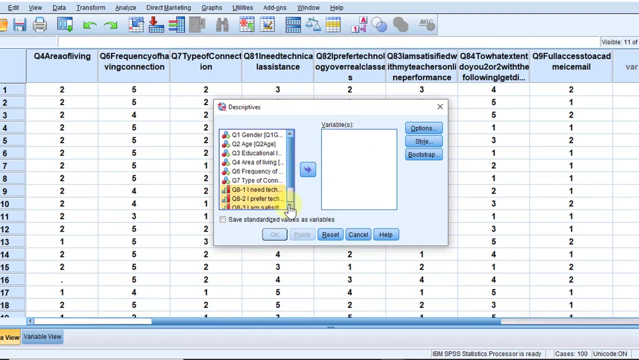 you the third method. so I'm going to go back to my spaces data view, go to analyze descriptive statistics, descriptions and then, the same way, I'm going to undo this to show you how I did it. so I'm going to select the statement. so I already I have just four statements, this scale going to: 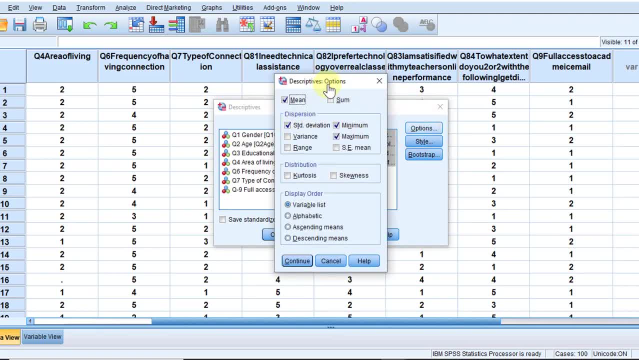 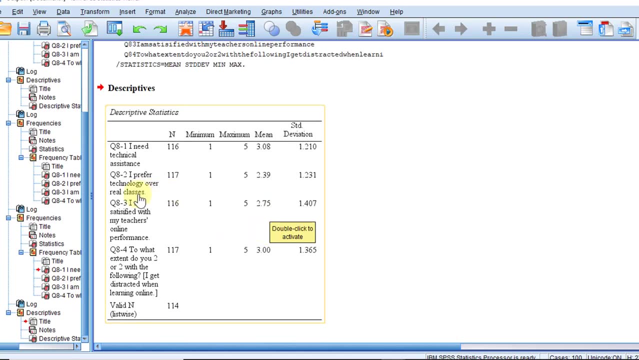 move them to the variables view, go to the descriptive, choose mean, standard, deviation, minimum and maximum. so these are the three types of data that I would like to have on the output and then click OK. so, as you can see, you have the four statements in this table. so my data or spaces tables are: 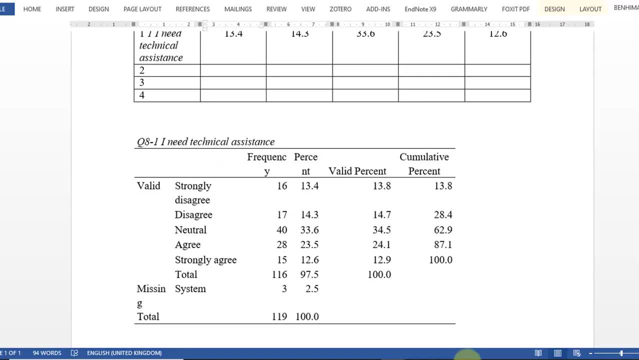 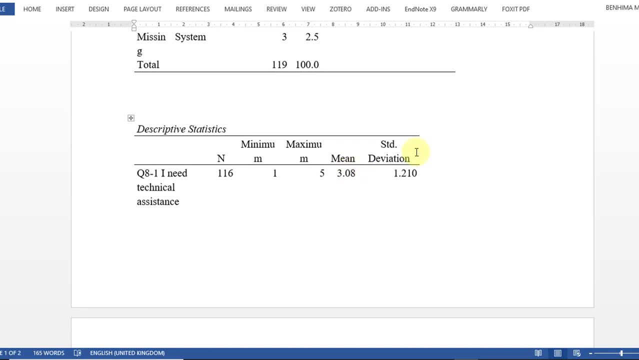 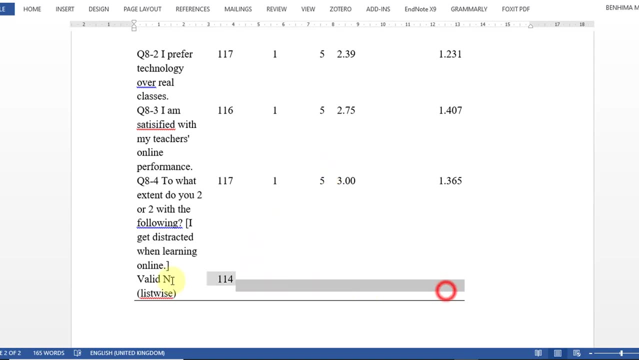 already formatted in APA styles. I'm just going to copy and paste this table here and interpret the results. I already have a video to interpret results on the basis of the mean and there are some argumentations on that. but in the literature you can you can find references that consider record data.